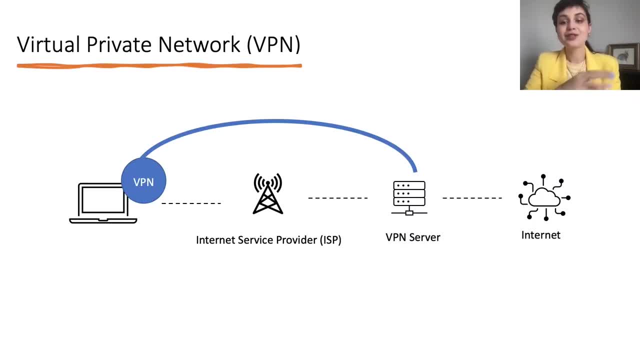 So let's start with the introduction, So just to make sure we're on the same page. in theory, virtual private networks create a secure encrypted connection- or a tunnel, as you can see- to a server from which users can access destinations on the internet. 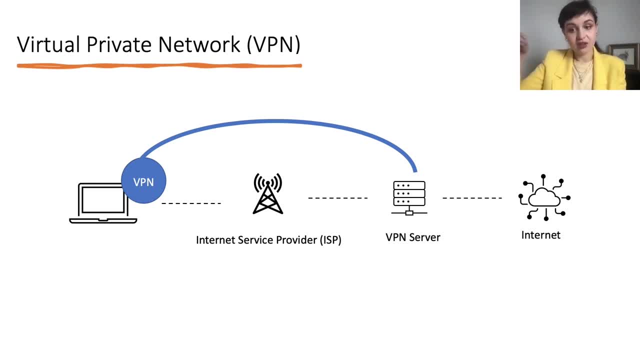 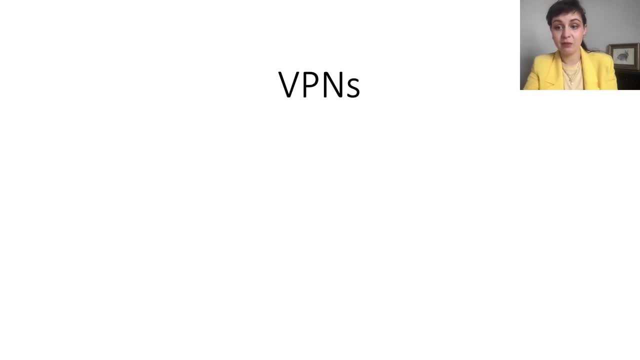 So basically, it seems that the user connects to the internet from the VPN And on the VPN server, and then we usually call that the user's Internet Service Provider, And there are different kinds of VPNs, which can generally be divided into two groups. 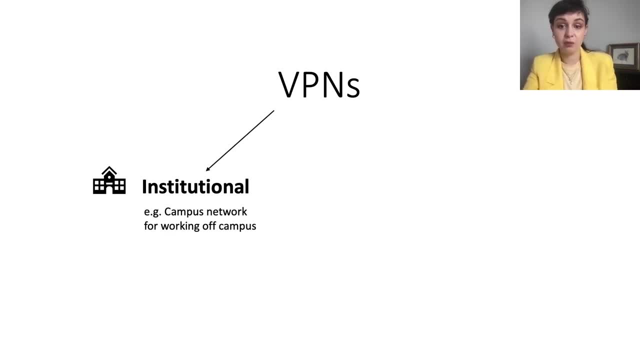 Institutional, which was actually the first intention for VPN usage. These VPNs are used in certain institutions, organisations, corporations or universities. They enable users to access destinations on private networks, like private enterprise or campus networks. So, for example, I use Global Protect when working from home or travelling. 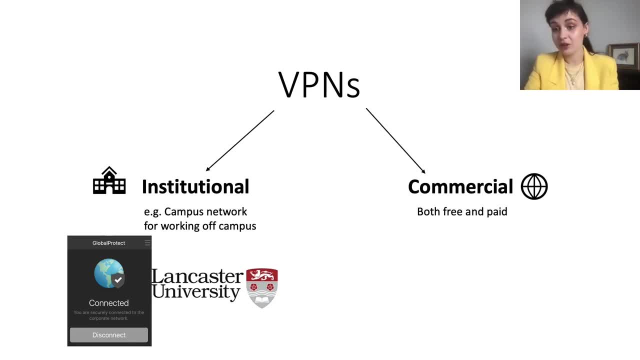 cannot be at the office. On the other hand, commercial VPNs are not used for any particular institution. Those usually commercial VPNs, especially paid ones, have different servers in different locations for users to choose from. So, for example, they can access the content that they are interested in And some of 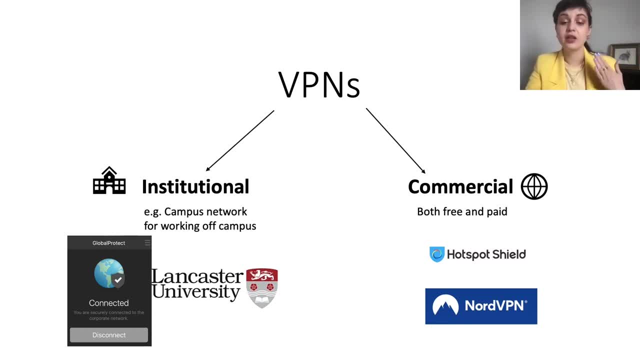 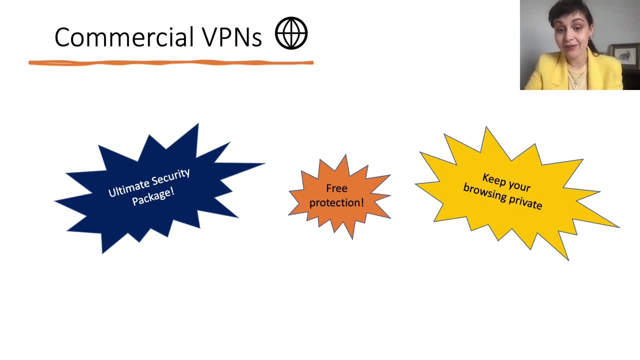 the most popular VPNs among our participants were Hotspot Shield and NordVPN, And actually in many cases, commercial VPNs adversely use themselves as privacy tools. However, recent studies show that VPNs can leak traffic and be susceptible to attacks. So, actually, their ability to provide 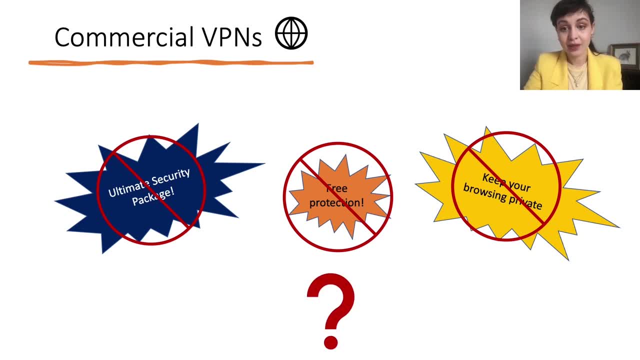 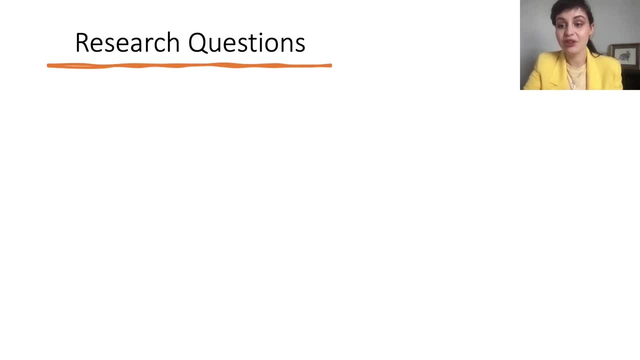 anonymity might be limited, But do VPN users know about these risks? So this led us to create three research questions. Why do people use VPNs? Are people aware of the security and privacy risks of VPNs? Why do people use VPNs? Are people aware of the security and privacy risks of VPNs? 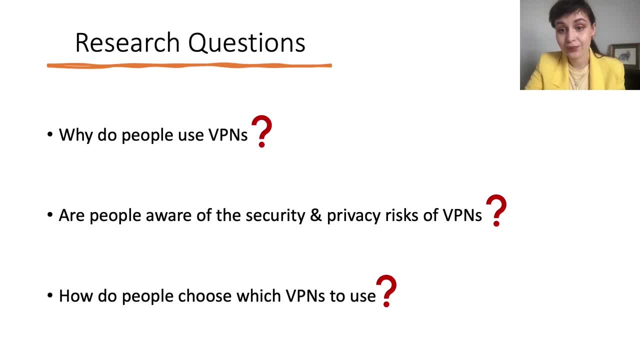 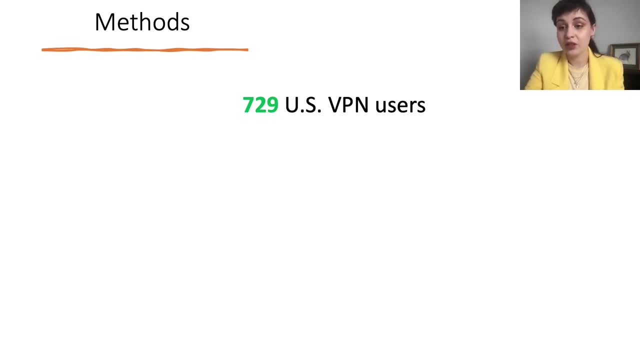 Why do people use VPNs, Are people aware of the security and privacy risks of VPNs, And how do people choose which VPNs to use? So this takes us to the methodology that we used. We conducted a two-part study of 729 US users in total In one part of the study. 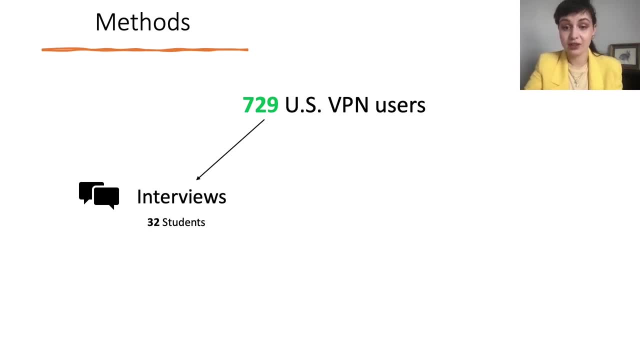 we interviewed 32 student VPN users from one university in the US. Twelve of them were from the US and 20 participants were international students. We also conducted a survey of 349 students from the same university as the interviewer. We also conducted a survey of 349 students from the same university as the interviewer.